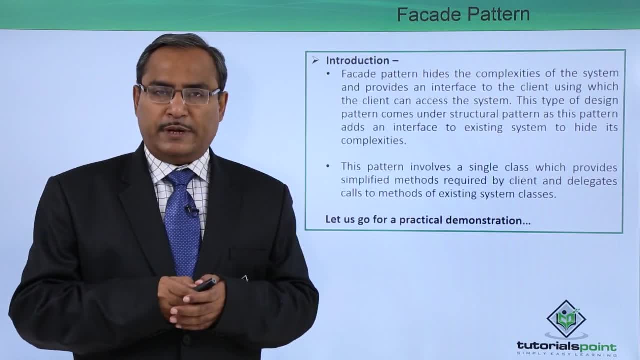 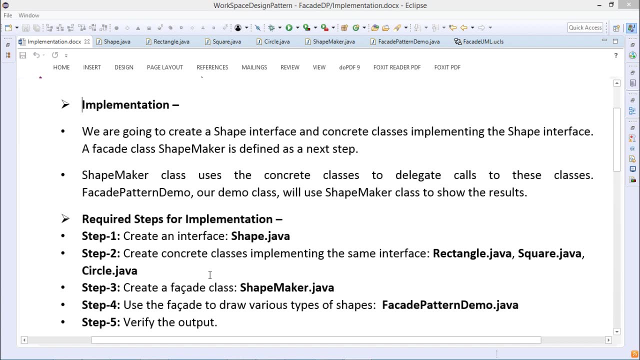 better understanding and implementation of facet design pattern. So here is a demonstration for you. In this session we are using Java programming language. We shall go for the implementation of facet design pattern. So we are going to create a shape interface and 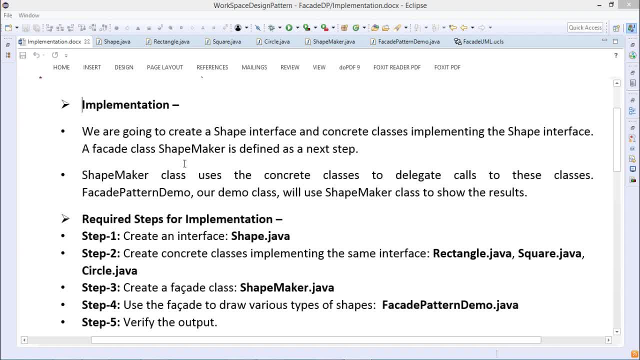 concrete classes, which will be implementing the shape interface, and a facet class that is a shape maker. So this shape maker class uses the concrete classes to delegate calls to these classes. There is a facet pattern. demo will be about demo class, which will use the shape maker. 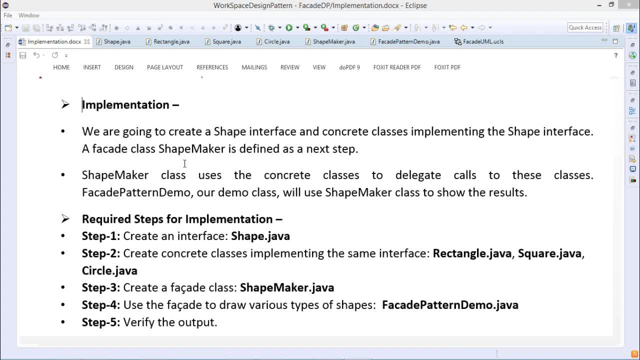 class to show the required results, to have the better clarity on this particular planning. So let us go step by step. So at first we are going for create an interface, that is the shapejava. So this is our shapejava. So now it is very simple that we are having this. 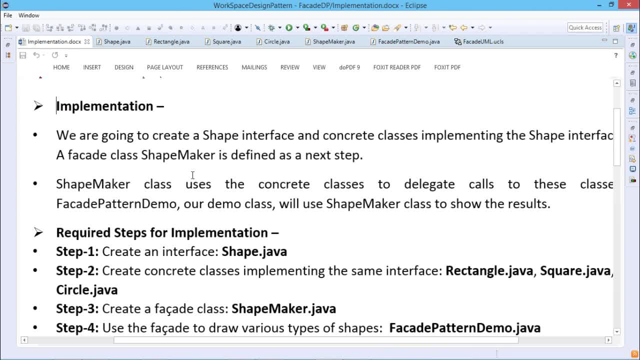 interface, shape, which is having only one method, that is draw here. So next one is that create concrete classes implementing the same interface, that is, a shapejava. There is a shape interface and here the concrete classes will be rectanglejava, squarejava and circlejava. We know that in. 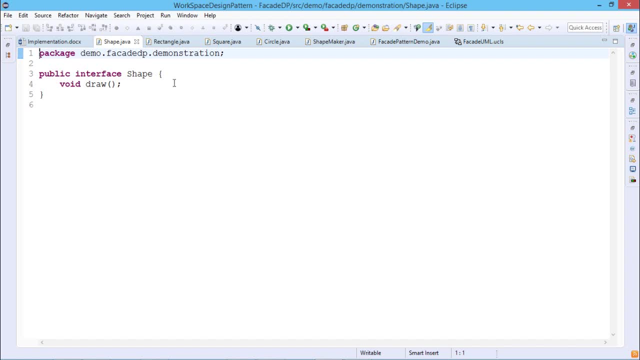 case of shape interface, we are having one unimplemented method, that is a draw. So in case of rectanglejava, we are just overwriting and implementing the method draw. You can see the code. and similarly we are doing the same in case of squarejava. So in case of 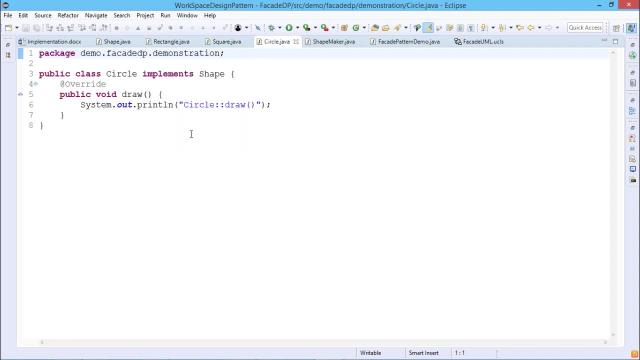 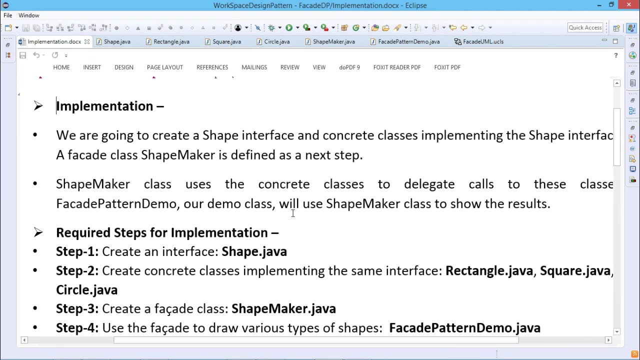 square and also another implementing class that is the circle, implementing the shape interface. So public void draw, systemoutprintln circle, colon colon draw here. So this is our interface and this is our implementing classes. Step number three: create a facade class, that is a shape makerjava. So here we are having. 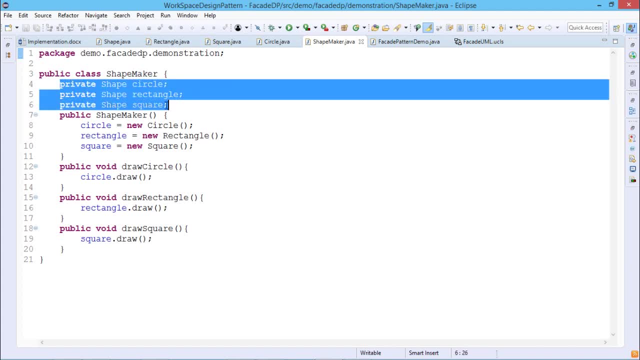 the shape makerjava. Here we have defined three private shape objects: that is our circle, rectangle, circlejava and squarejava, And this is our shape maker constructor. So the class name is shape maker and this method constructor method is also shape maker, as is well. So in this shape, 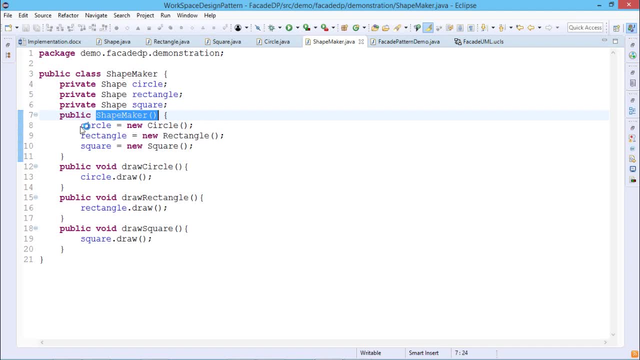 maker, constructor. we are just instantiating this instance- variable circle, rectangle and square- using new circle, new rectangle and new square. So respective constructors will instantiate this respective objects. We are also having another one that is a draw circle. We are having anotherjava. 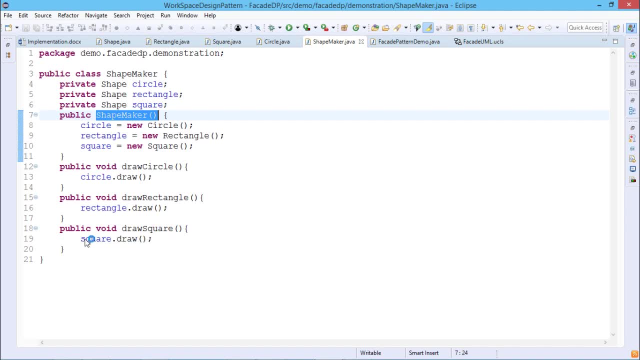 method: draw rectangle. We are having another method, that is a draw square, So circledraw, rectangledraw and squaredraw. So now you see, in case of rectangle, we are having this draw method overwritten. We are having this square also, in case of circle also, And this 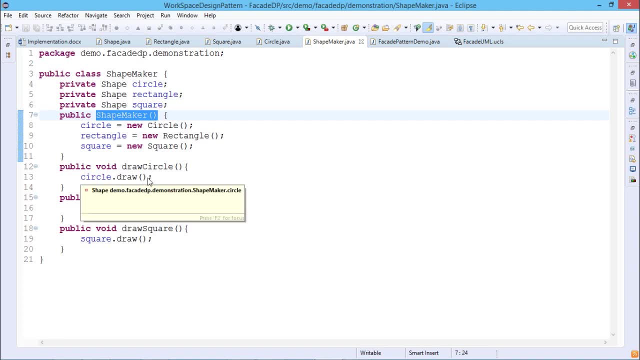 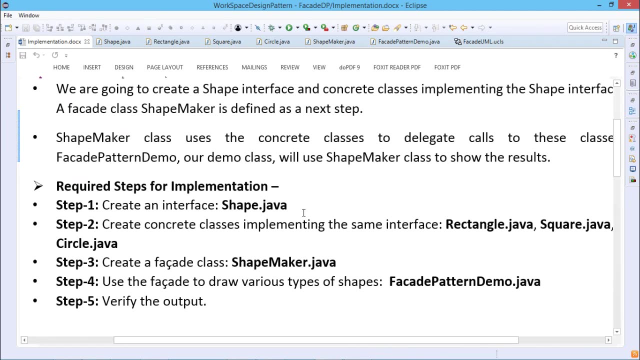 is our shape maker, where this circle class objectdraw will execute this method as usual. So now we shall go for our step number four. use a facade to drawjava, Yukosahabóyótypesjavajff. All as we perform our researchcom Seniltly these. 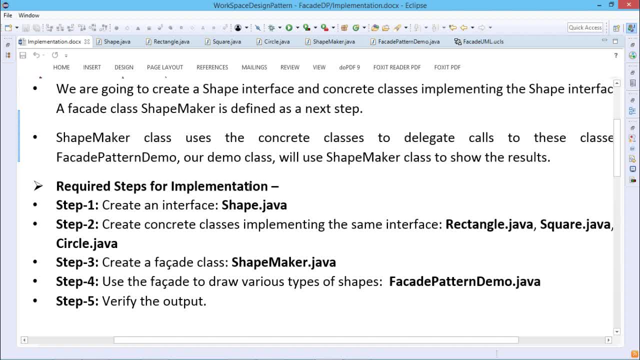 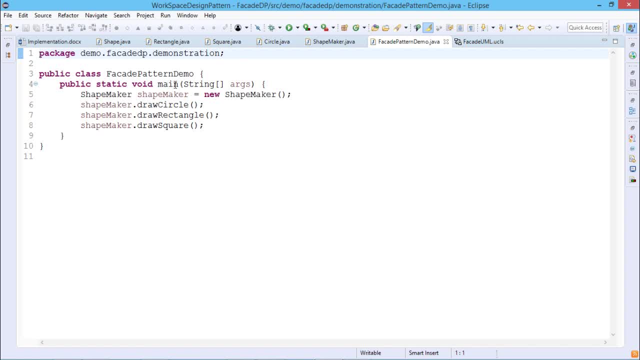 models are audiojava, not audiochipJava. HCизtqúsicaagóas undowho, sir всí at a namespeakcom Very useful. And then we have another: waterfalljava &java, javaPattern et al step5.. Let us start. 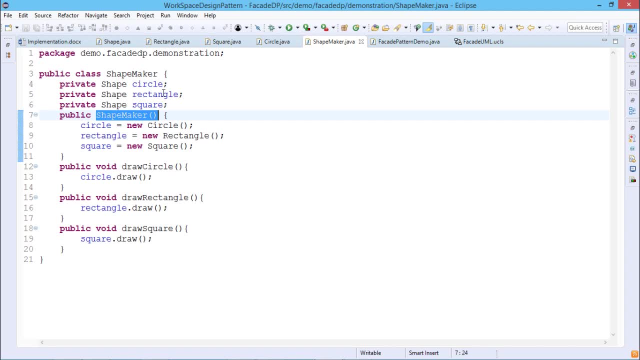 and this particular private shape circle, private shape rectangle and private shape square. these are the three instance variable as they are under the private scope, so they are remaining and inaccessible from the outside world, but using this draw methods which are under this public section. so now the circle dot draw, rectangle dot draw and square dot draw can. 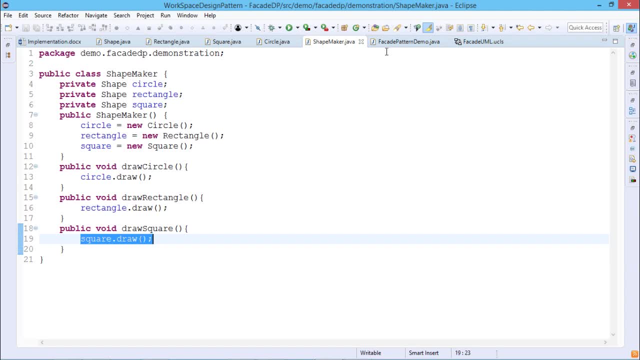 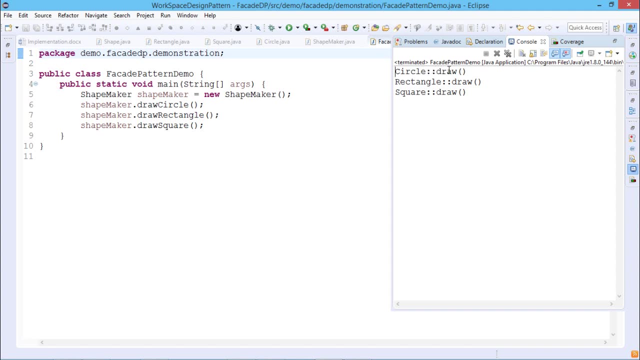 easily be accessed within this from this class shape maker. so this is a facet pattern demo, so let us go for the execution of the same. you can find that circle- colon colon draw. rectangle colon colon draw, and square colon colon draw. the respective strings have got printed, which. 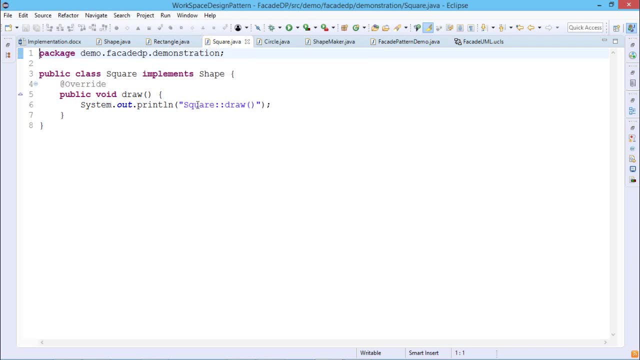 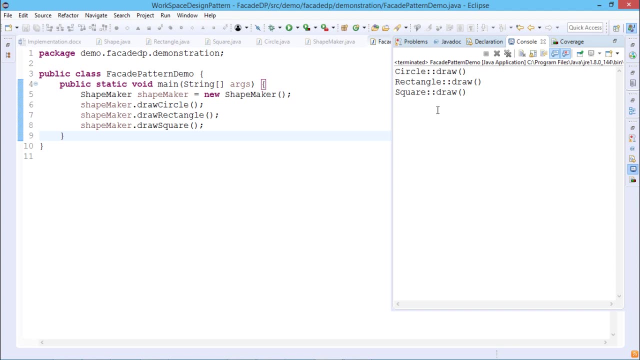 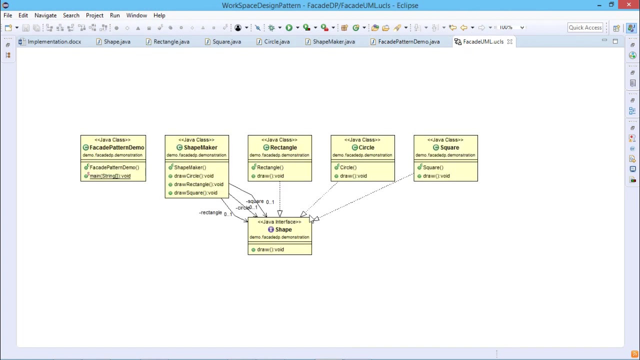 were there written here in this particular rectangle, square and the circle. so this is a facet pattern demo. you are getting this output very much logical and you are getting this idea how this facet design pattern can be implemented. so now let us go for the class diagram. so let us go for the class diagram. 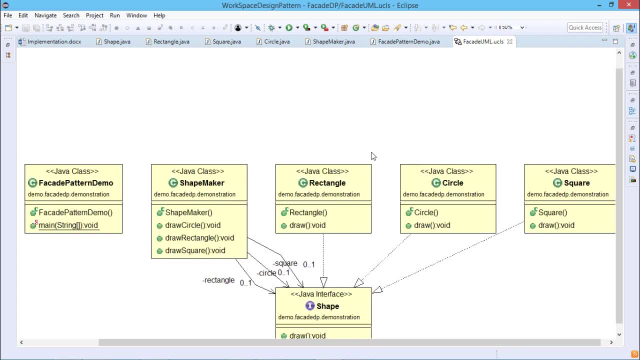 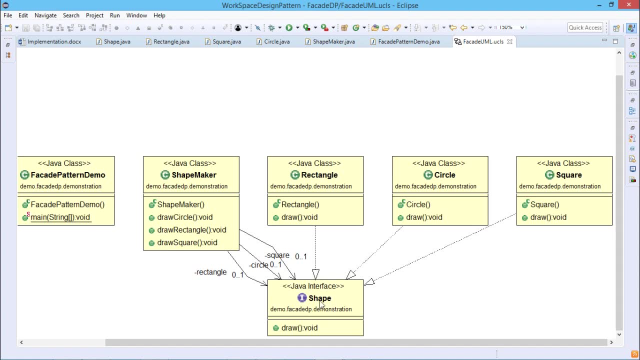 let us go for the class diagram. i'm just zooming a little bit. so this is the class diagram we are getting. so here we are having this shape. this is the interface. it has got implemented in the classes, that is, the rectangle circle and the square. and here you see, we are having the shape maker. we are having the shape maker, so this particular